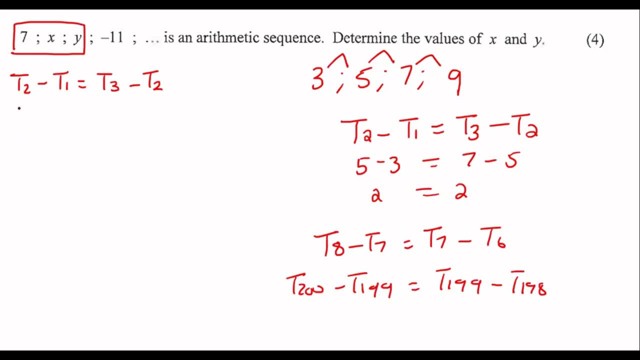 7 minus x. I mean x minus 7.. x minus 7 is equal to y. Then you could simplify that a little bit if you wanted to. It would eventually say that 2x minus 7 is equal to y. Now don't panic, There's nothing you can do there. So what we do is we go on to the 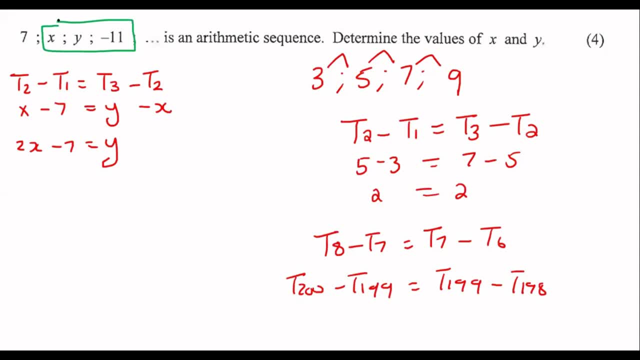 next one. So we use this, We can use these three, So we can say that term 4 minus term 3 must be the same as term 3 minus term 2, for example, So that would be minus 11.. Minus y must be the same as y minus x. I'm then going to simplify a little bit. 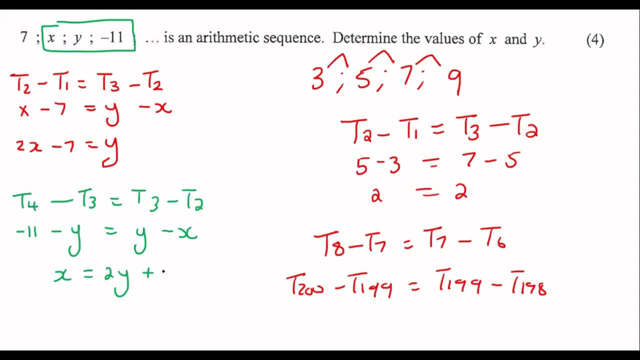 You should eventually get: x is equal to 2y plus 11.. You can do it in another way, but that's just. yeah, that's the way I saw straight away. And then, of course, we just use simultaneous equations, And so simultaneous equations can. 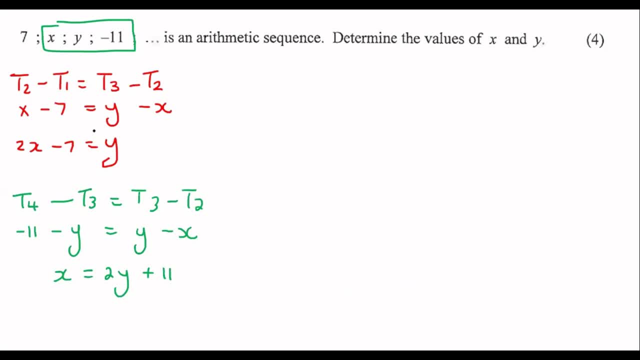 be done in many different ways, But what I'm going to do is: you see this equation here. It says that y is equal to 2x minus 7.. So what I can do is I can replace this y with 2x minus 7.. 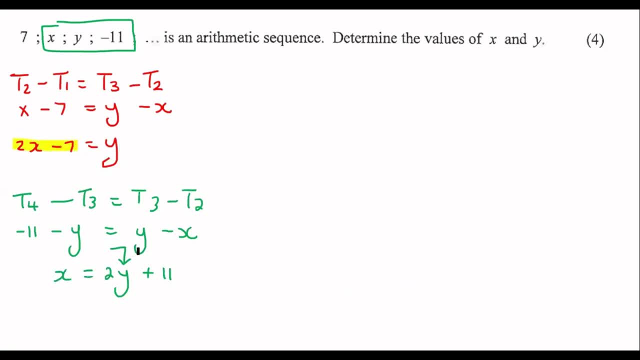 Let me show you guys what I'm talking about there and there, See, I'm going to replace that y with 2x minus 7.. And so what that would look like is the following: So we can say, okay, wait. 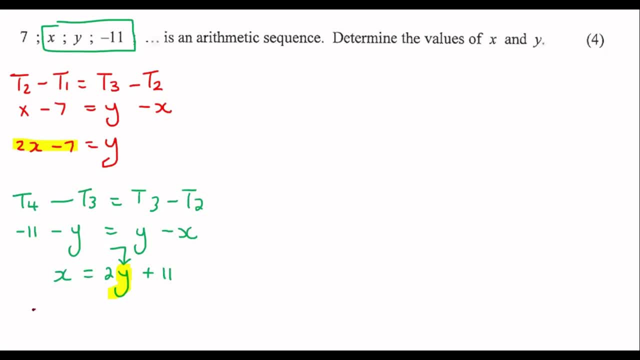 let me just change my color here, Red, So we can say that x will be equal to 2 times 2x minus 7 plus 11.. And so x will be equal to 4x minus 14 plus 11.. And so, if you eventually solve this, we should find that 3x will be equal to 3.. 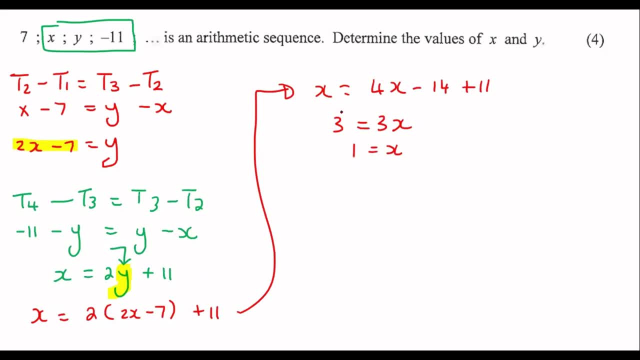 And so x will be equal to 1.. We can then put that, we can put that 1 over here, And so that will allow us to find y. So we can see that y will be equal to 2 times 1 minus 7.. 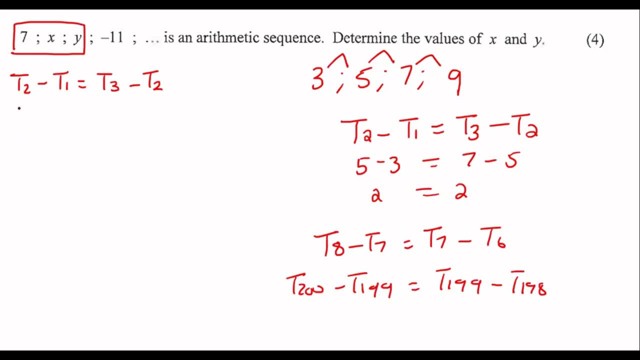 7 minus x. I mean x minus 7.. x minus 7 is equal to y. Then you could simplify that a little bit if you wanted to. It would eventually say that 2x minus 7 is equal to y. Now don't panic, There's nothing you can do there. So what we do is we go on to the 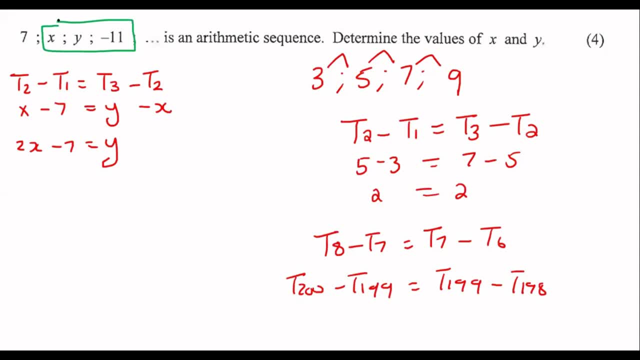 next one. So we use this, We can use these three, So we can say that term 4 minus term 3 must be the same as term 3 minus term 2, for example, So that would be minus 11.. Minus y must be the same as y minus x. I'm then going to simplify a little bit. 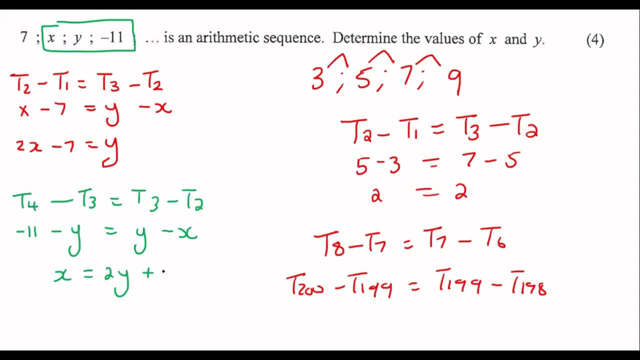 You should eventually get: x is equal to 2y plus 11.. You can do it in another way, but that's just. yeah, that's the way I saw straight away. And then, of course, we just use simultaneous equations, And so simultaneous equations can. 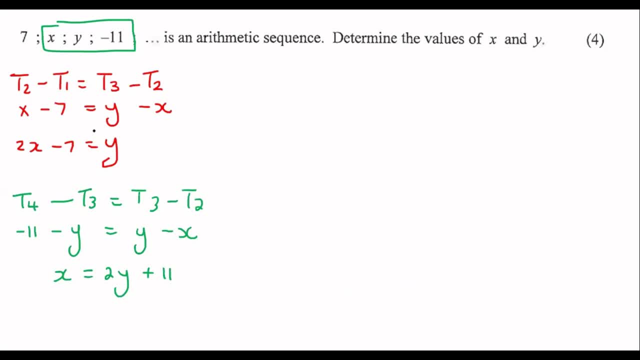 be done in many different ways, But what I'm going to do is: you see this equation here. It says that y is equal to 2x minus 7.. So what I can do is I can replace this y with 2x minus 7.. 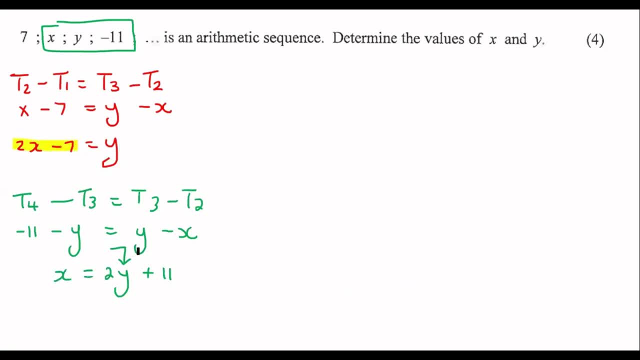 Let me show you guys what I'm talking about there and there, See, I'm going to replace that y with 2x minus 7.. And so what that would look like is the following: So we can say, okay, wait. 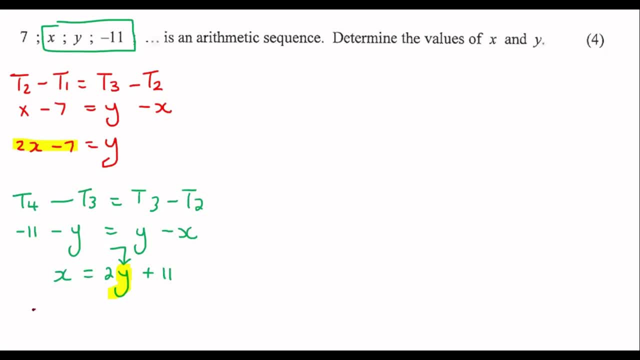 let me just change my color here, Red, So we can say that x will be equal to 2 times 2x minus 7 plus 11.. And so x will be equal to 4x minus 14 plus 11.. And so, if you eventually solve this, we should find that 3x will be equal to 3.. 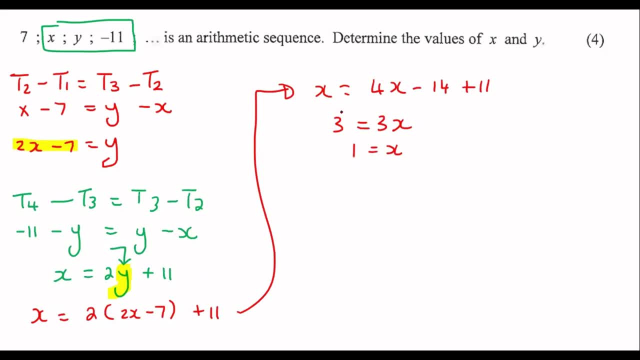 And so x will be equal to 1.. We can then put that, we can put that 1 over here, And so that will allow us to find y. So we can see that y will be equal to 2 times 1 minus 7..